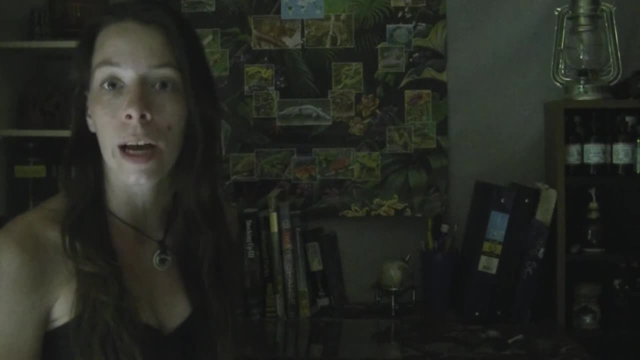 because you didn't pay attention to what the leaves or the roots look like, or anything to that effect. So the first thing that we're going to start off learning through this subject is how to identify leaves. over anything, Leaves can be the first thing that you look at to make sure that you have a 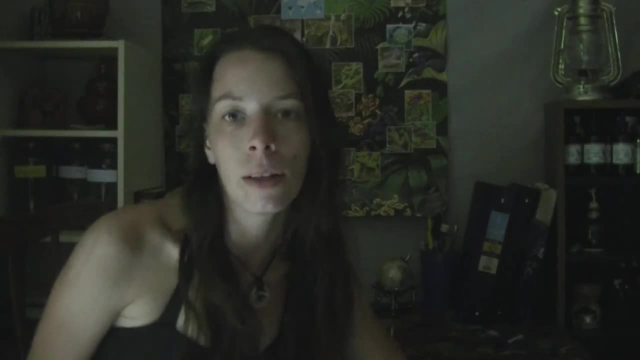 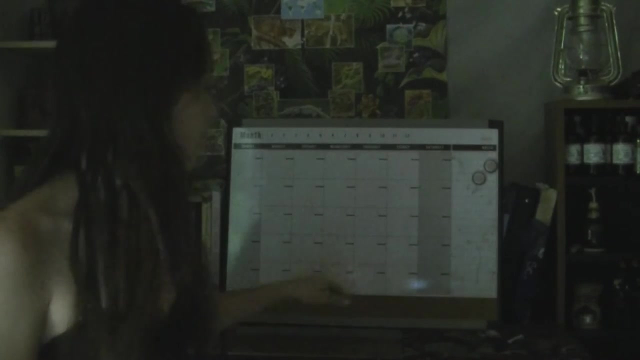 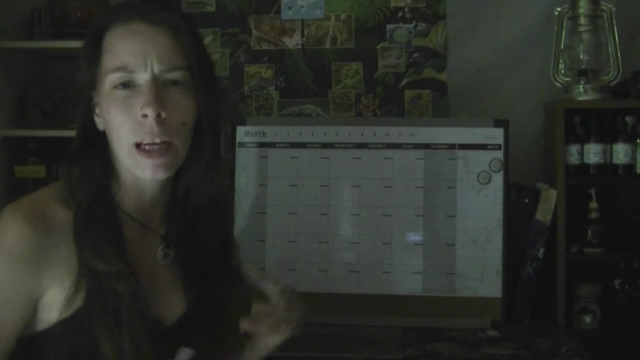 proper identification. So I'm going to pull out my little whiteboard here and I apologize that it is a calendar, but that's what I have right now and I don't want to waste the paper. So the first thing we have to do is know the parts of our leaves. I'm not going to go into cell structure. I may make 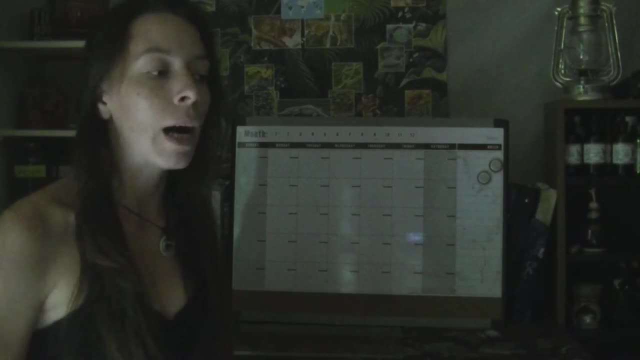 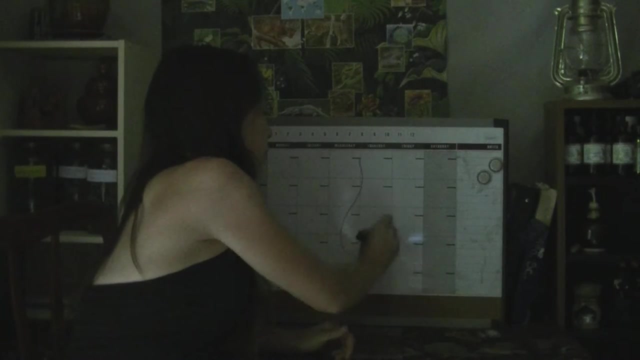 another video on that for people who really want to get into it, but I'm just going to do basic parts of the leaf from when your looking at it. So if I draw a simple leaf with my awesome artistic skills, you have a few different main parts of your plants that you'd want to know. 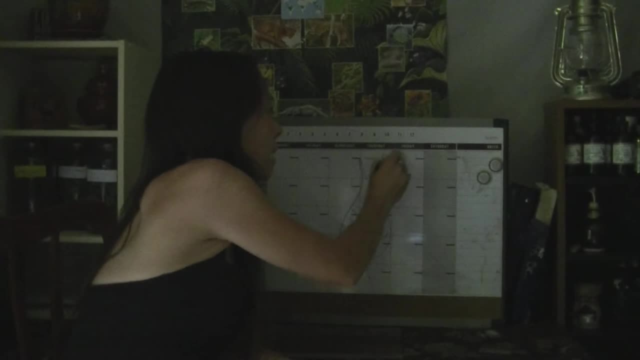 The very tip of your plant is what's called the apex a-p-e-x. then you have what's called the margin of your plant, which is the edges of it, just like the edges of your paint are your margins. Margins can be wavy, or they can be spiky, or they can have teeth. 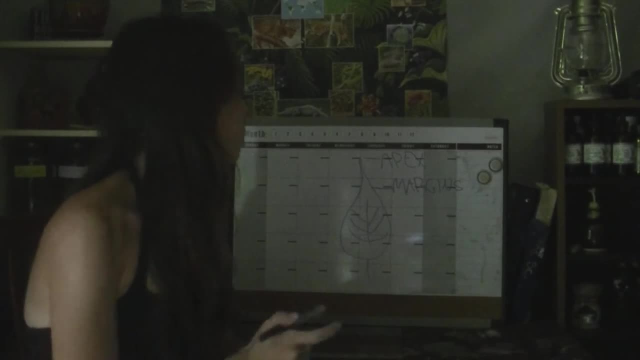 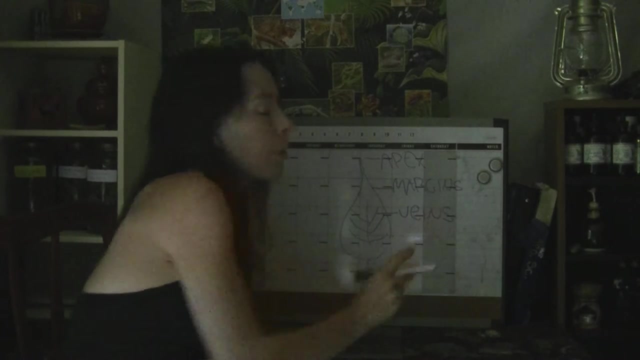 or they can be smooth, or etc. Then you have your veins. Your veins are those small indents that are all through your plants, just like the veins in our skin. Those are your veins. and then you have the base of your plant. All leaves will 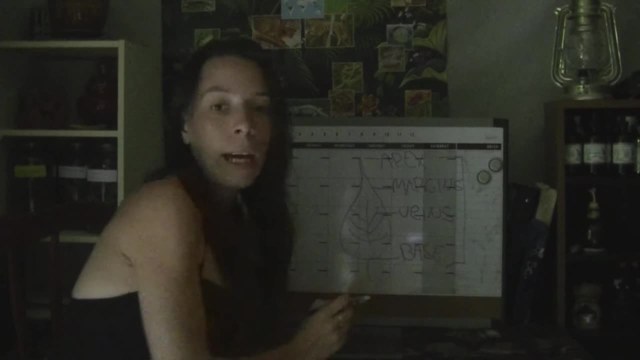 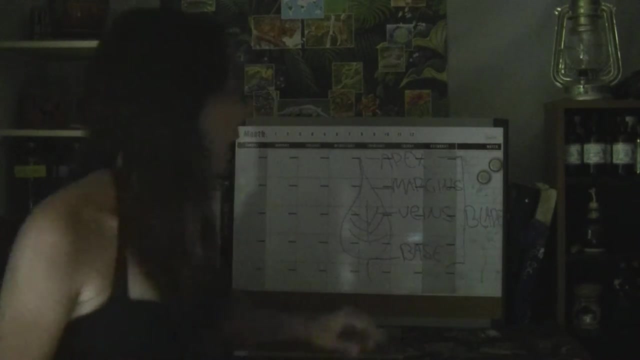 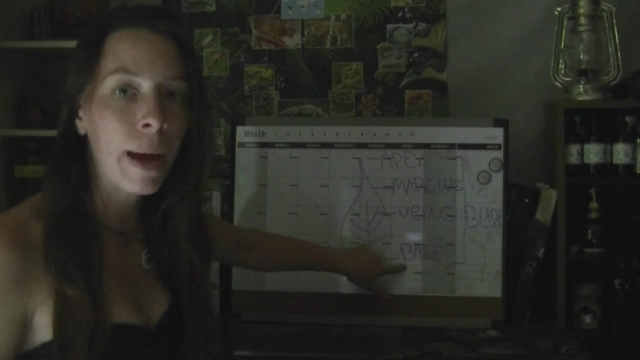 have these four structures and put together. these four structures are called the blade. So you have the blade, which consists consists of your apex, your margins, your veins and your base. Then plants have a few other structures that some leaves may have and some leaves may not have. The main one is: 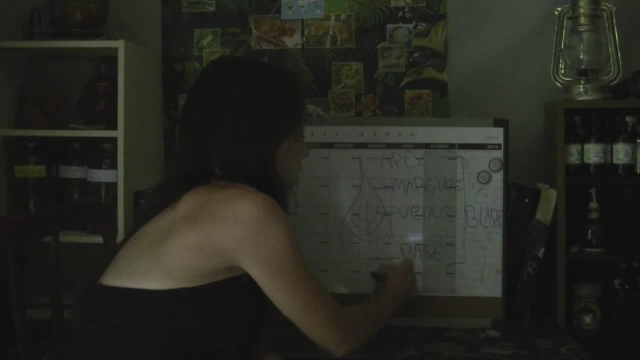 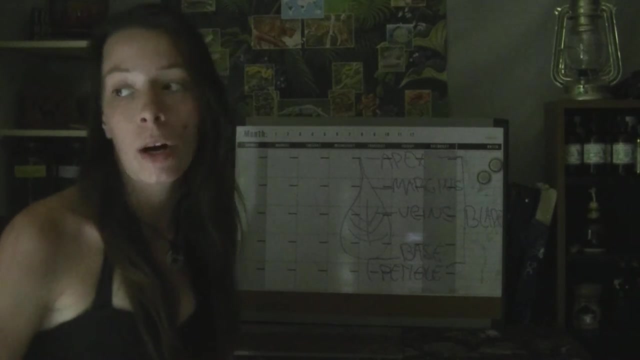 called the petiole. It's P-E-T-I-O-L. The petiole is pretty much the stem of the leaf. A lot of people see and they believe that, oh, that's a piece of the plant itself, of the stem of the plant itself, but it's. 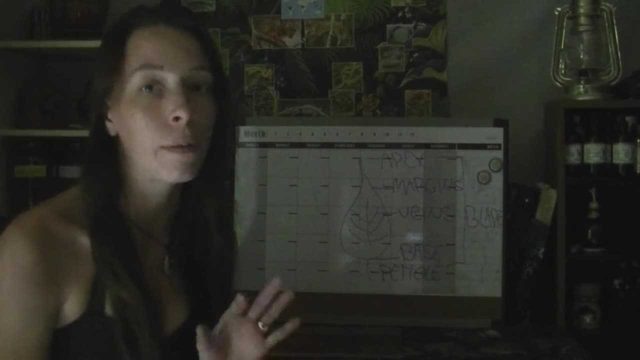 not, It's the stem of the leaf. So when you pull an oak or maple leaf up off the ground and it has that little woody stem on the bottom of it, that's actually called a petiole. A petiole can be flat, it can be short, it can be long, soft round it can. 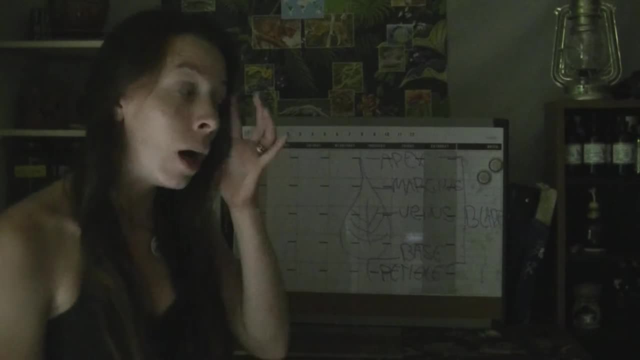 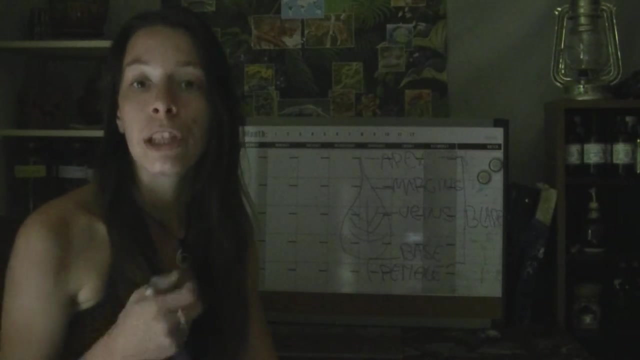 be shiny, not shiny: wood like, plant like, etc. A good example for you to understand how much of a variation there is and what a petiole may look like: When you're eating celery, that stalk that you're eating is actually the petiole of the stalk's leaves. Now if 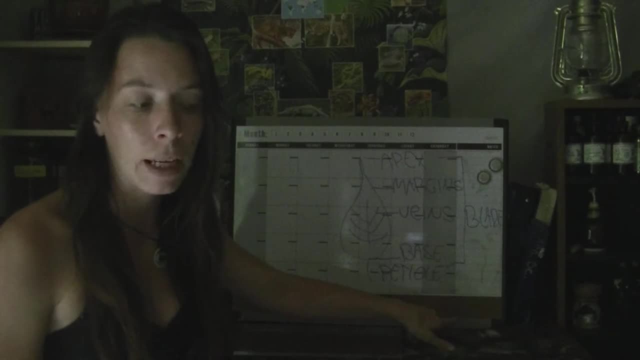 you have a plant that does not have any sort of a petiole. a good example of that is bananas, birds of paradise trees, anything like that, where that leaf almost acts like a sheath to the stem of the plant and kind of grows right out of it with no stem. that would be. 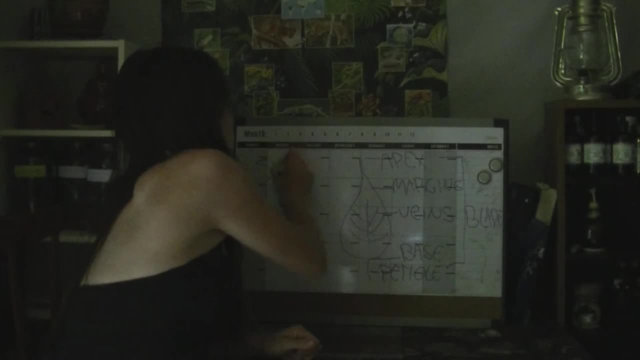 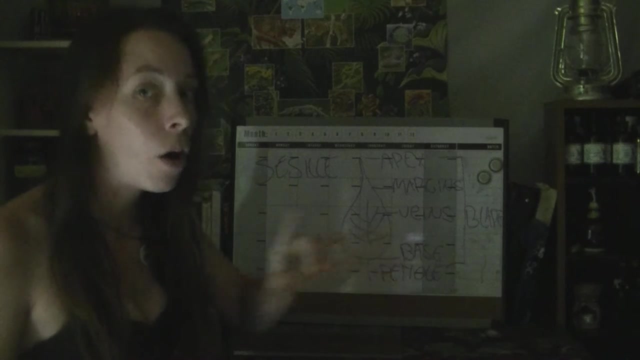 called a cecily. It's s-e-s-i-l-l-e. a cecily plant. Sometimes- again, not all plants have these, but some do that. when you look at the bottom of the petiole, where it attaches to a plant, which is also where your axillary bud would be located, you may see two short 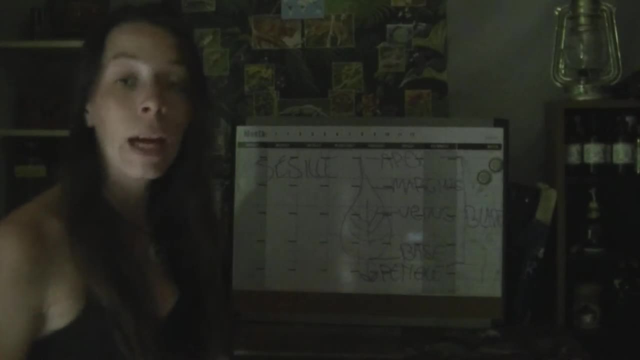 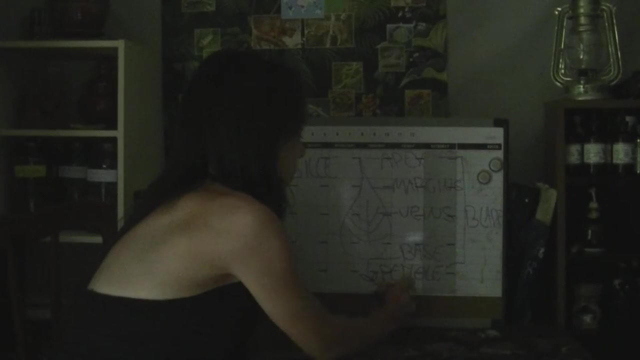 spiky leaves that that petiole is growing out of. if and again, if they don't all have this, if you see those leaves, that is called a stipple, s-t-i-p-u-l-e a staple. again, staples and petioles do not. 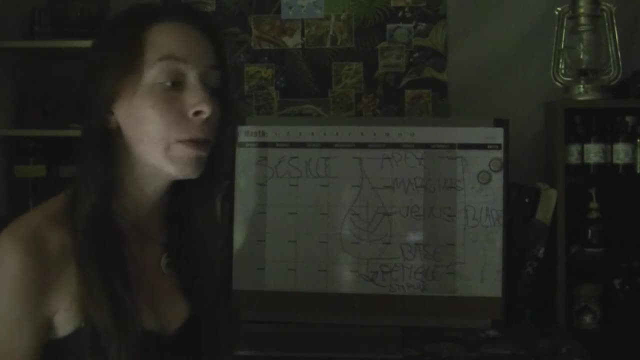 exist on all plants. but that is a good way that if you see a petiole, it may be able to say, okay, well, it's not this plant, because I know this plant doesn't have a petiole. So again, you have four main components that all leaves will have. 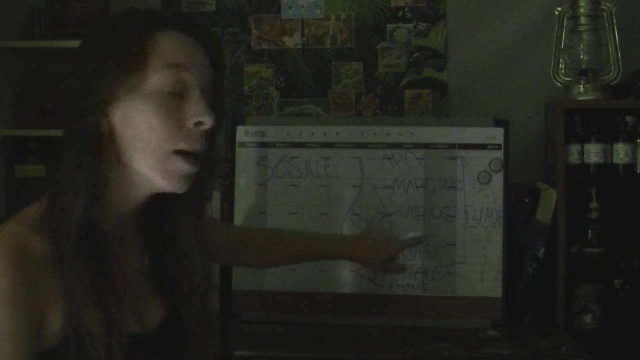 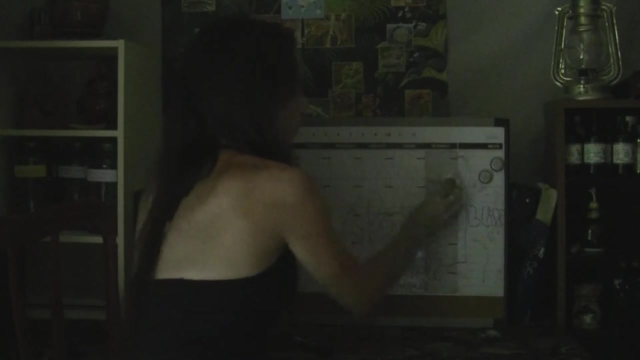 Your apex, your margins, your veins and your base. that creates the blade of the leaf, and then you may or may not have a petiole or a stipple. So if we grab my little eraser here, it's actually a piece of paper towel. 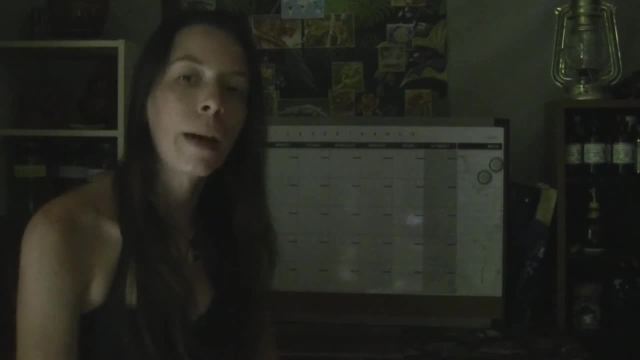 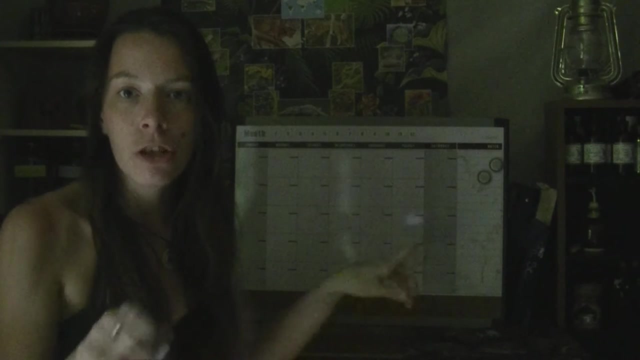 The next thing we have to learn is how these leaves come together on a plant, because you may have two plants. The both have petioles, they both have staples, the margins of the leaves are exactly the same, the veins are set up exactly the same and the only difference is is how those leaves 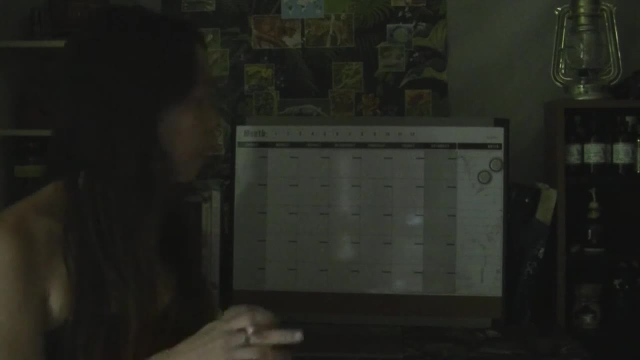 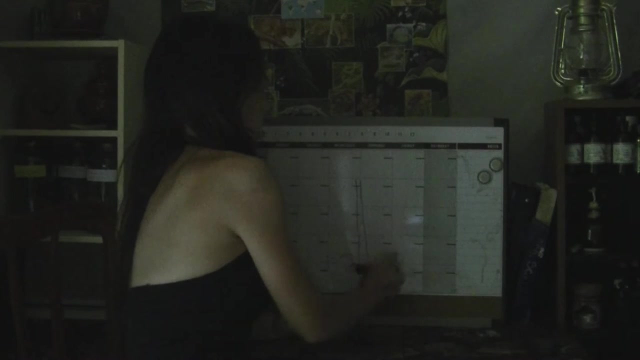 are compounded to each other, The first basic ones we have, which I'm going to throw a little flower here so that we can have an idea. we got the stem of our flower, we have the ground, we'll make it like it's in a little pot here and then we've got our flower at the top. it doesn't have to be a 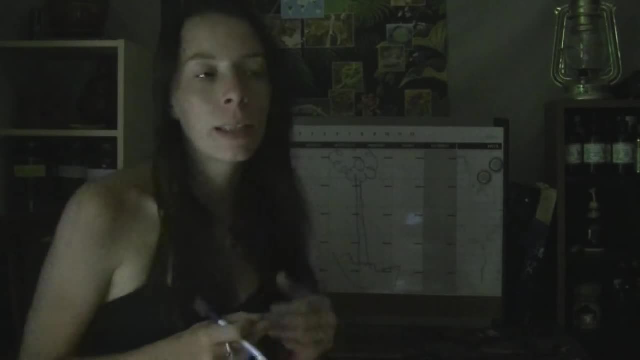 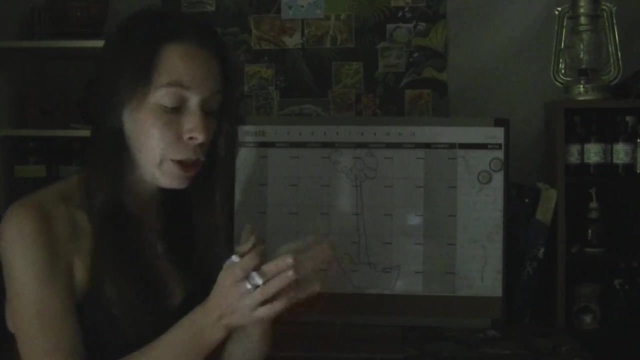 flower, Where the leaves of plants attach to the stem is always called a node and that is literally just the conjunction. you're not going to see a specific node. sometimes it will have a bump from where the stem is swollen to push the leaf out, but it's just where that leaf attaches. 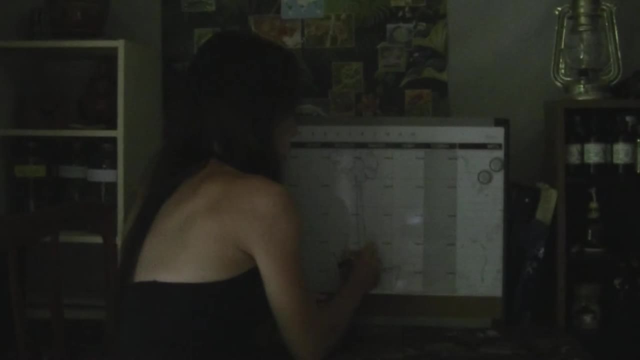 to the actual plant is called a node. So I'm just going to draw some little dots. they don't actually look like this, I'm just using it for reference along my plant. Then we'll call those nodes When a plant only has one leaf coming out of each node. so we'll draw a little leaf. 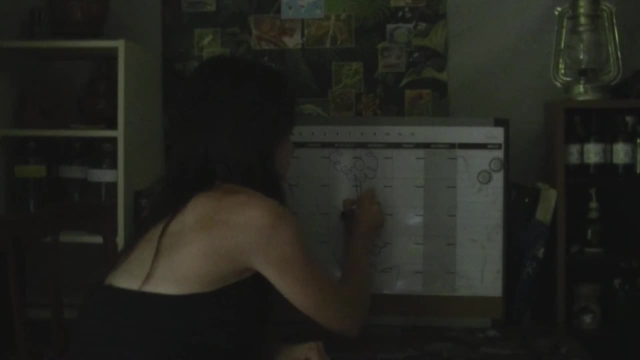 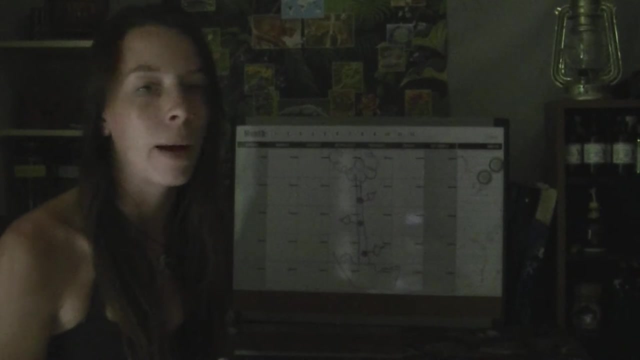 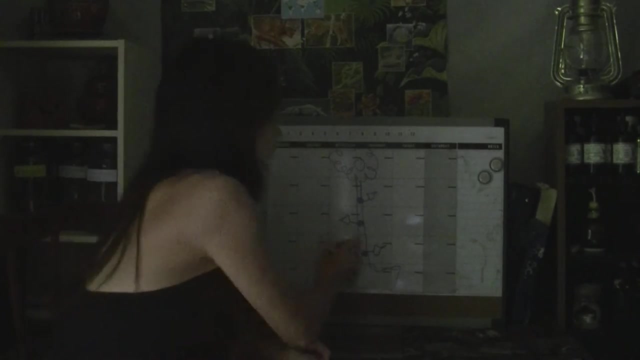 out of each node here on it's petiole. That is called alternating. it has an alternating compound of leaves. so now you have one, two, three, four. that's alternating. so when only one leaf is coming out of your node, that has alternating compound. If you have two leaves coming out of each node, so we'll put another. leaf out each side here. I'm just going to draw in these little triangles here. If you have two, and only two, leaves coming out of each node, that's going to be called an opposite compound. Think about it. leaves are facing opposite ways. sometimes they'll. be facing the same direction, but a lot of times they'll be opposite ways. so it's called opposite compound. Two leaves out of each node equals an opposite compound. Moving up from there, if you have more than two leaves, any number can be 3,, 4,, 5,, 6,, 7, whatever. 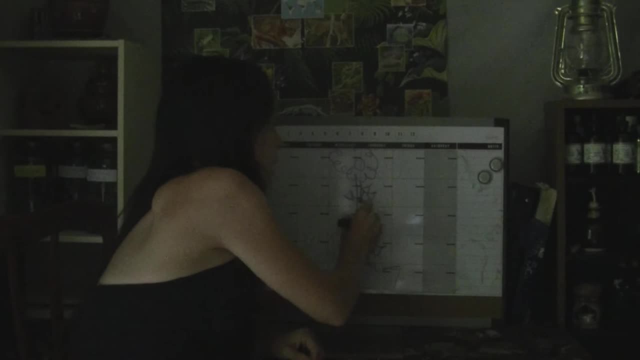 if you have more than two, two or more leaves coming out of each node, I'm just going to draw them each with three. that's what's called a Horeld compound. So it's going to be W-H-O-R-L-E-D. Think about it like. some people call it a Horeld compound, but it's. 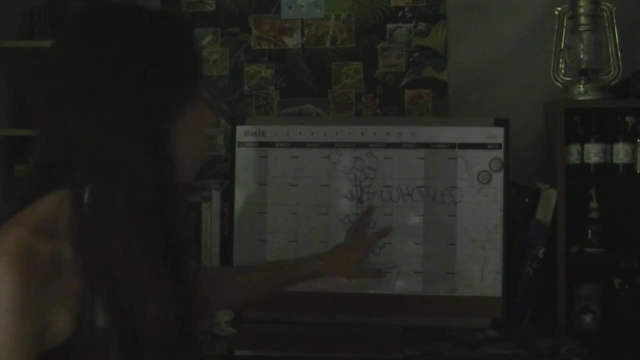 something that's whirling. the leaves are whirling around the plant, so you have more than two, not two, or more more than two, so three or more leaves coming out of one node. it's going to be called Horeld- What Horelds can move into, and this is where some 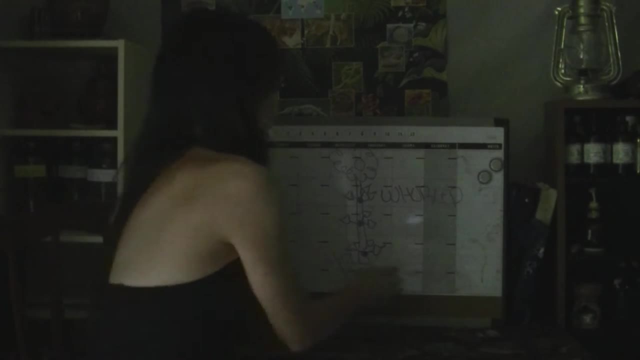 people get a little confused is that if we get rid of our plant here with all its Horeld leaves? if you have a plant, I'm going to draw a Dandelion, because Dandelions are very common. Dandelions are the best example here of something that most people will know. If 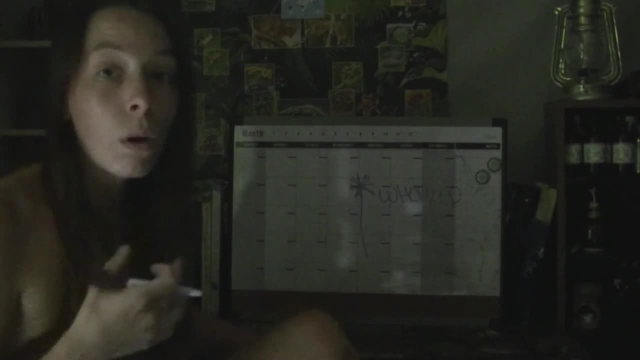 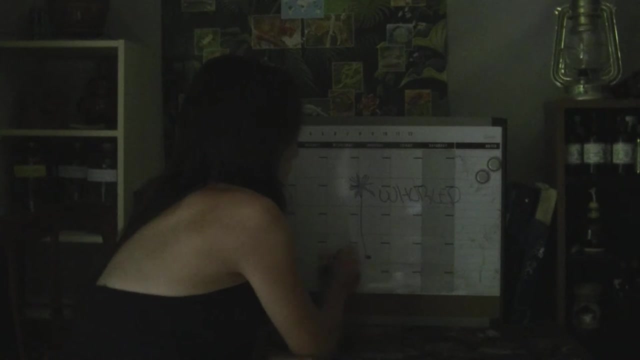 you have your Dandelion and you have a Horeld set of leaves, so again, three or more coming out of one node, but it's only coming out of the base of that plant. so here's our ground and you have three or more leaves coming from the base of that plant at the same node, so that the stem is growing out of that Horeld of leaves. you know it has leaves at the ground. it's going to be called a basal rosette. b-a-s-a-l-r-o-s-e-t-t-e. it's called a basal rosette. and again, that's only at the base of the plant. there would be no other leaves going up the rest of the plant. it just has a hoard of three or more leaves where it's coming out of the ground and then shooting a stem up. it's called a basal rosette. so those are the simplest compounds. of leaves. again you have your alternating, which is one out of each node. opposite, which is two out of each node, holy, three or more out of each nose node, or a basal rosette, where you have three or out of one node at the base of the plant. to get a little more clear-cut. it's called a basal rosette and when you look at the elements around your plant when you use a basal rosette, you'll see that you can see that the整料 Onyx is teaspoon complicated. we're going to get into some pinnately and palmetly compounds. The pinnately: 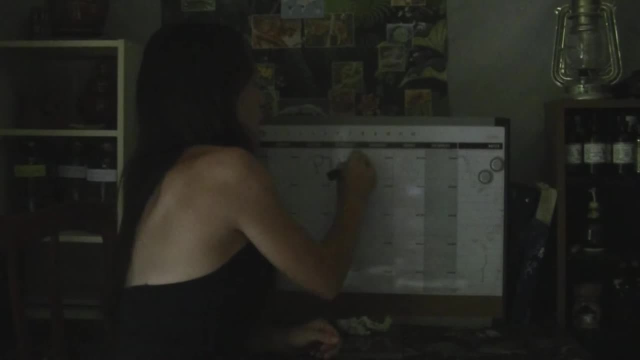 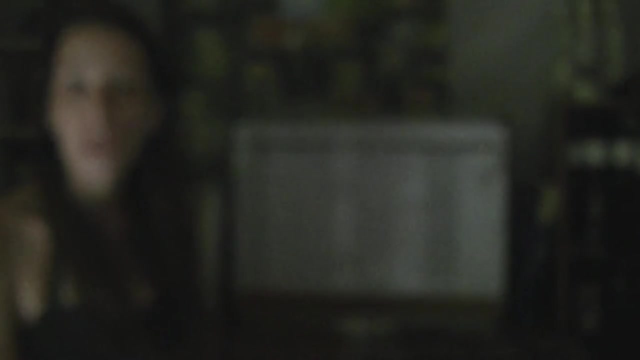 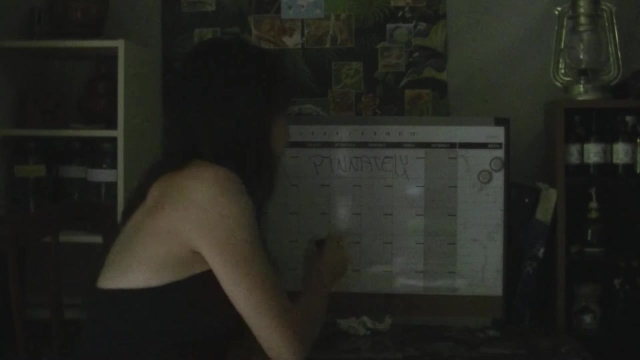 which is P-I-N-N-A-T-E-L-Y pinnately compound, is something you'll see in fern-like plants. I'm trying to think of other examples off the top of my head. Fern is probably the best one, But that's where if I have my main plant and I have a petiole coming out of my plant. 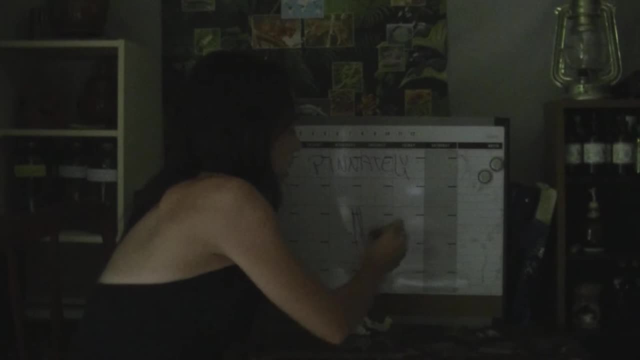 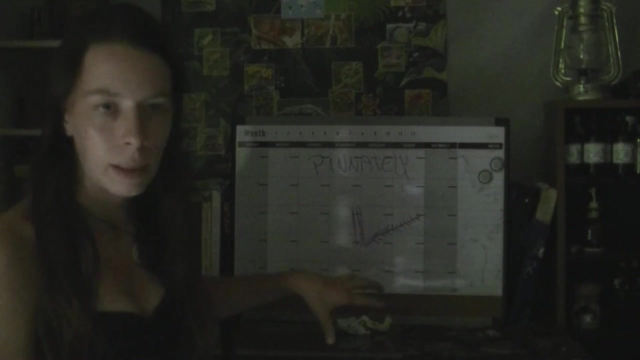 we'll call that a petiole. and the petiole continues to extend nice and far and you have tons of little leaves. I'm just going to draw them as lines coming off that petiole. it's going to be called a pinnately compound. But what happens? this is where it gets a little more. 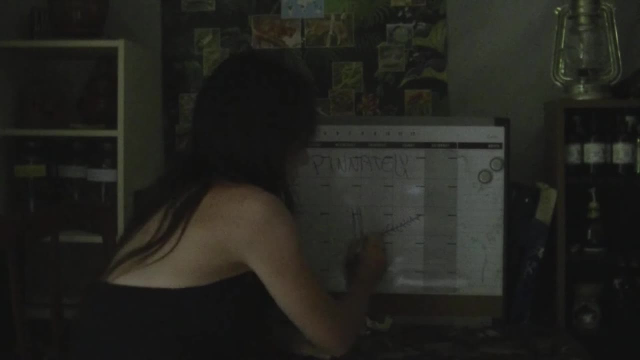 confusing and a little more in-depth is that petiole. the petiole ends where your leaf starts. we're going to draw a line there before all our leaves. Only this area would be considered to be the petiole. What it then turns into is what's called a rachis. it's R-A-C-H-I-S is where that. 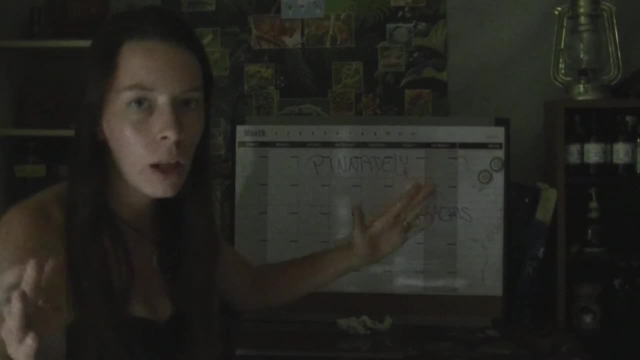 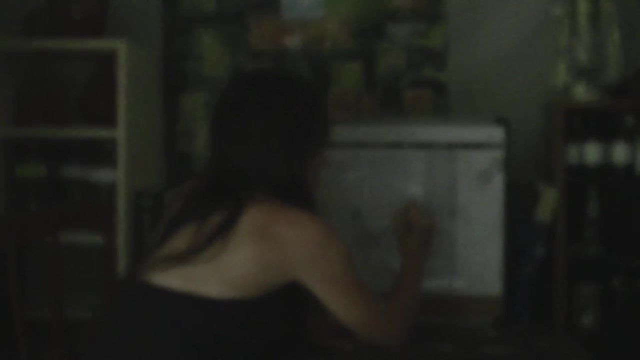 petiole continues way on nice and long. you know it technically would be short and long, but it has tons of little tiny leaves coming off either. I'll draw those more as leaves here. So you've got leaves coming off all over the place of this. thing, little leaves, That's going to be considered to be a pinnately compound. Then you have what's called a twice pinnately compound, and so you have your petiole again. it turns into your rachis, but then this rachis has rachises coming off of it. 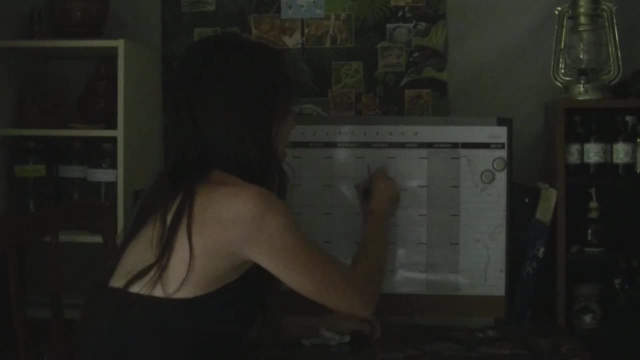 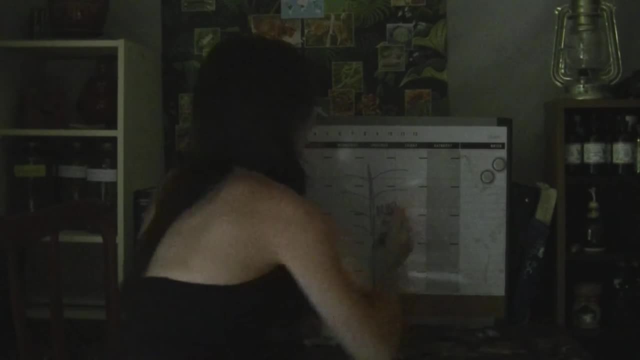 I'll do this fast so you can see it here. And it'd be like that: off, all these side shoot rachises. So you're going to have a main rachis right here and then all your side ones that are going to have 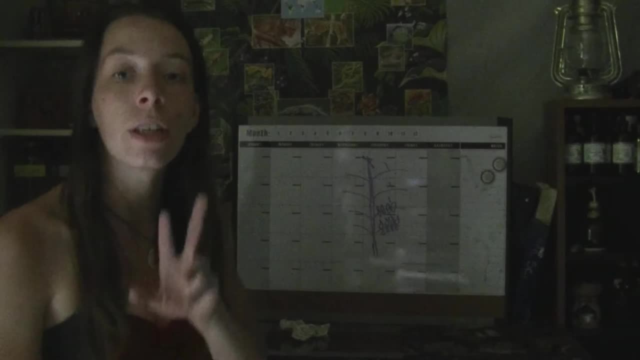 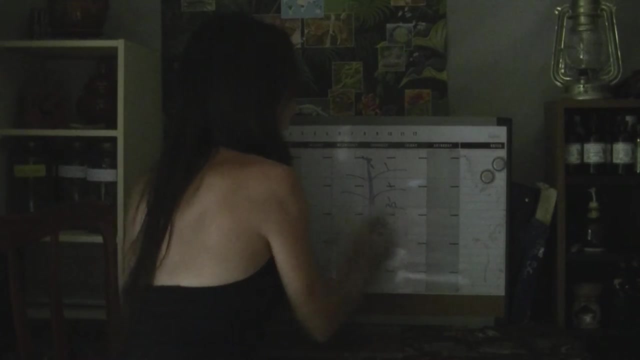 your leaves off of it. That's still a pinnately compound. it's just a twice pinnately compound. So it's pinnatelys coming off of pinnatelys, pretty much. From there we have what's called a palmetly compound. It's going to be P-A-L-M-A-T-E-L-Y, a palmetly compound. 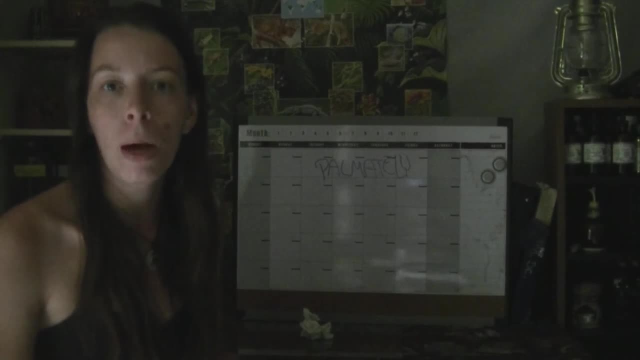 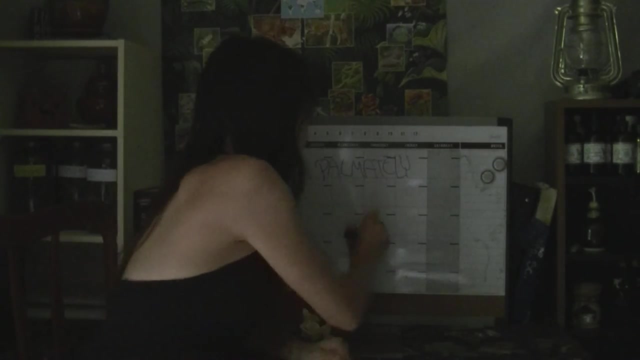 and it's kind of going to be like a Japanese maple leaf. It's going to be a palmetly compound. It's where you have what looks like multiple individual leaves, but it's actually one where these leaves are all coming back to a center base. 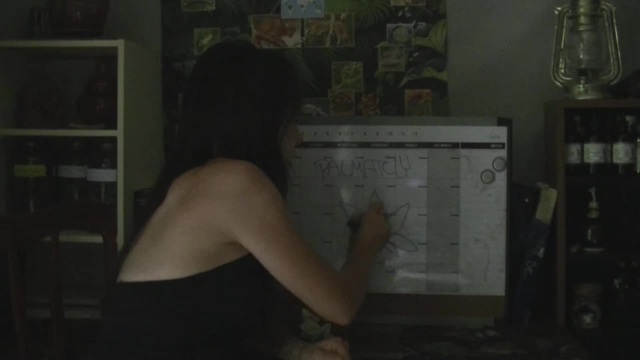 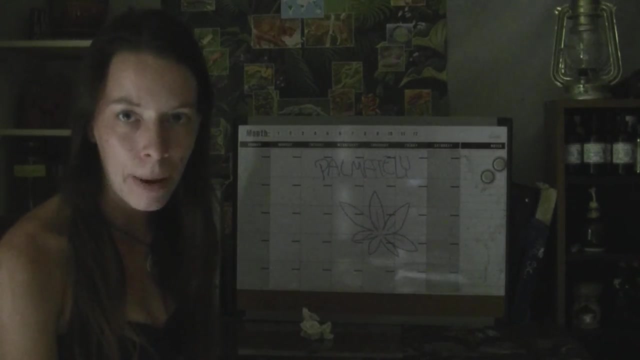 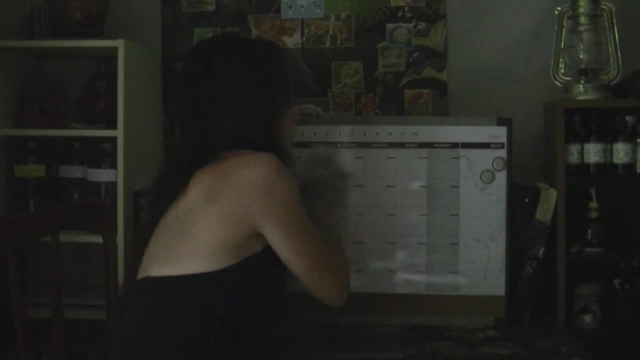 Kind of like drawing a pot leaf here, Like a center base with its own veins, and it ends up kind of looking like a hand. That's called a palmetly compound, So that's a pretty easy one to remember. So those are your main compounds of how leaves come together. Again, you have alternating opposite: palmetly, pinnately and twice pinnately. Those are all the ways that your leaves are going to come together. Now that we know how our leaves come together, we need to know how to define the margins of each leaf. 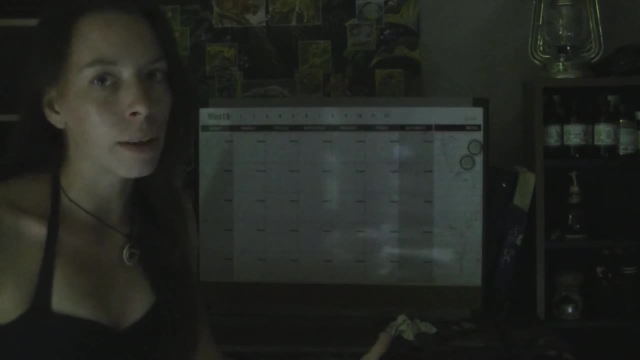 I'm gonna go, I mean you can go, I mean you can go, I mean you can go. go on forever about all the different types of leaves, but I'm gonna do your main different five types. the first and easiest would be called entire when you 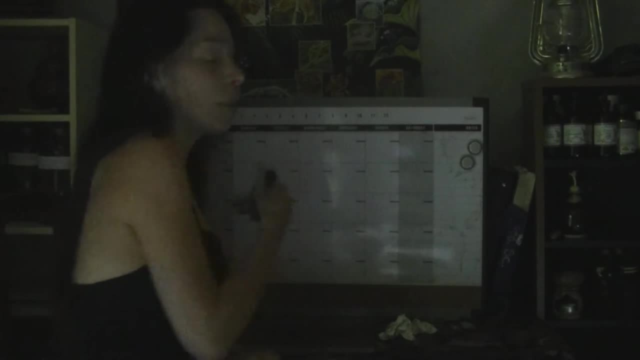 have an entire margin. it's just like the word entire, ENTIRE. that just has a very smooth margin. just your normal leaf, nice, smooth, unserrated margin. the next one is what's called a sinuate. it's s-i-n-u-a-t-e a sinuate. leave a sinuate. 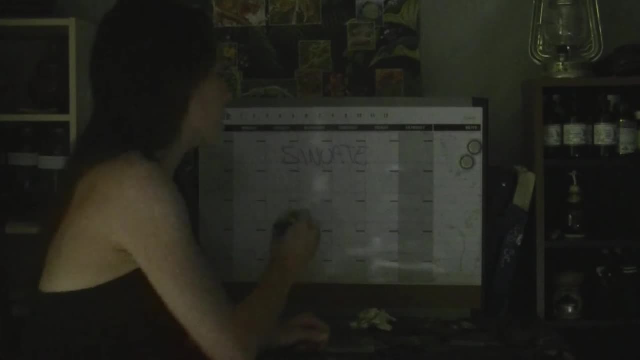 leave is where your margin is still smooth, but it's slightly wavy. so you're gonna have something like that. I mean, obviously neater than that, but still a very smooth margin. it's not jagged, it just has slight curves and waves to it. the next one is called your dentate. that's d-e-n-t-a-t-e. a dentate is where. 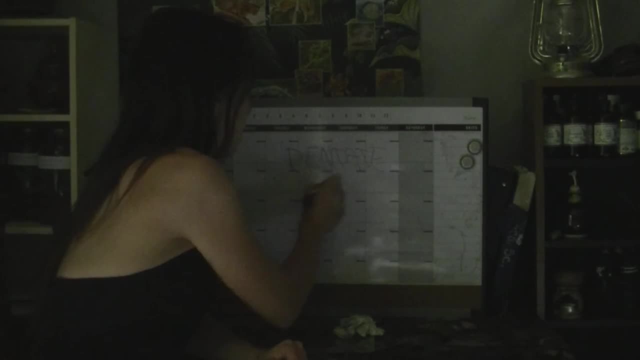 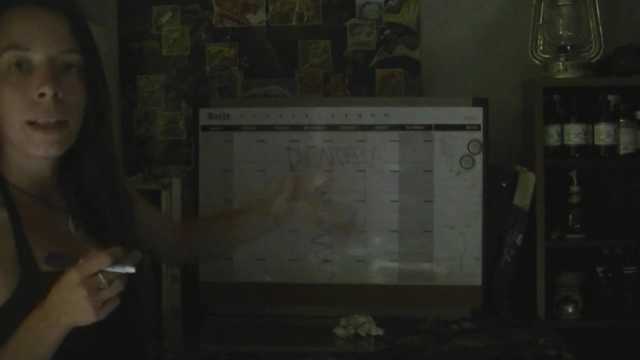 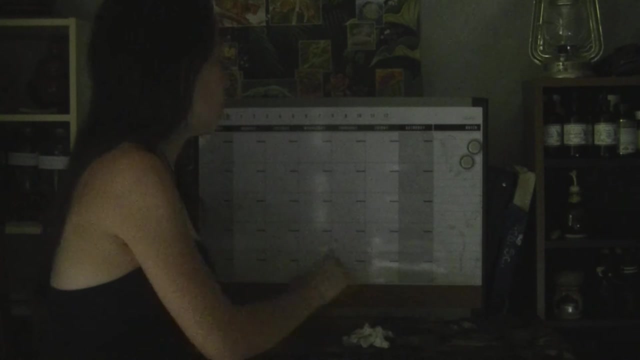 your margin has small outward poking teeth to it, so think about it like a jagged line. if your margin looks like that, it's called dentate. again, the margin is the edge of the leaf. then you have your dentate, what's called a serrate. your serrate is very similar to your dentate. it's gonna. 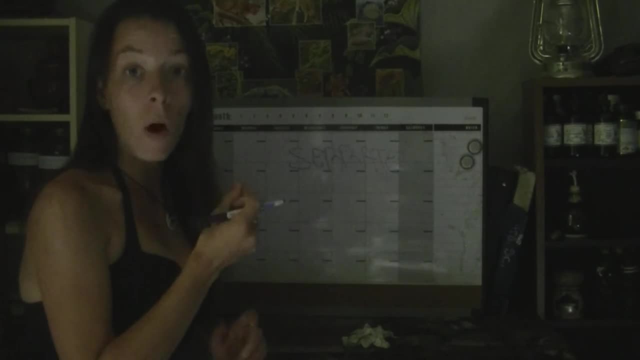 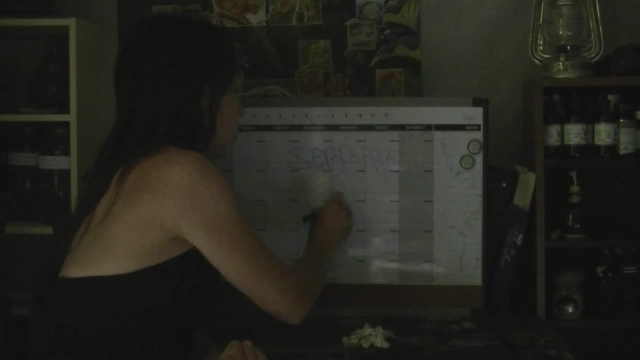 have teeth all along it, but your teeth are smaller and usually curving one direction or the other, kind of like a saw blade, so it's gonna look more like that. that would be a serrate. excuse me, after serrate you're gonna have what's called. lobed. lobed is similar- excuse me- to your sinuate jeez. I'm losing my words, I apologize. lobed is similar to your sinuate geez. I'm losing my words, I apologize. lobed is similar to your sinuet, but it's more defined. 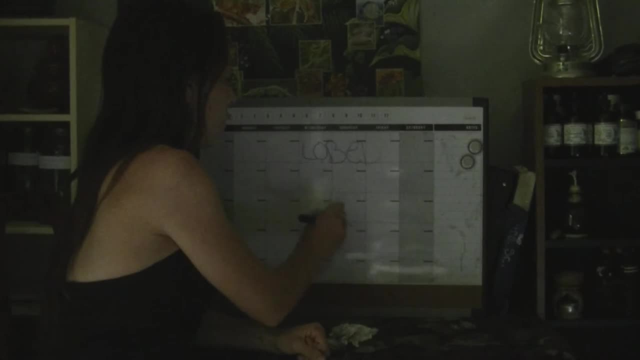 your lobes are kind of going to come all the way out and back in and all the way out and back in, all the way out and back in, kind of like you would draw a cloud. that's your lobed. well, just so that you can remember the difference: your sinuet is still smooth and it just has very slight wavy curves to it so that you can see the difference: lobed versus sinuet. so those are your main five different types of marginal structures. okay, after all that, we're going to go over two more ways to identify your own leaf type, and the first is by shape. the first shape: you have. it's called elliptical. elliptical is just basically an normal size oval, normal proportions of width to height, etcetera, and it's just the shape of an oval. the next you have is what's called the lanceolate. lanceolate, which is L? A N C E O L A T E lanceolate. 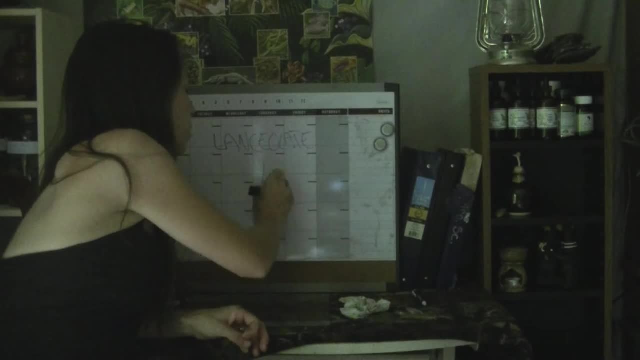 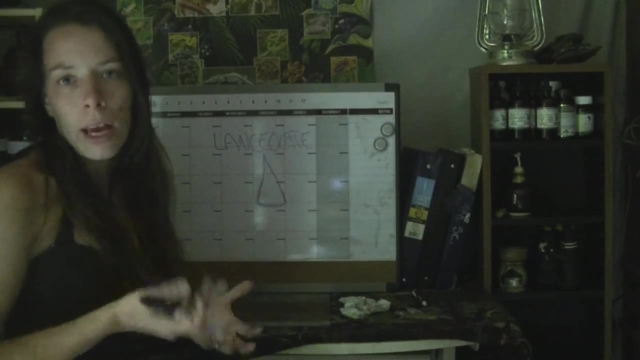 it's pretty much the shape of a triangle with a nice point at the end slightly curved bottom. the way I like to remember that one is Lancelot. It kind of looks like the tip of a spear or maybe a sword or something to that effect. So I think of it, Lancelot. The next one is: 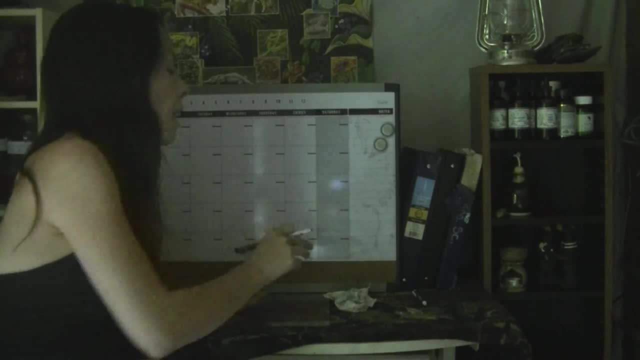 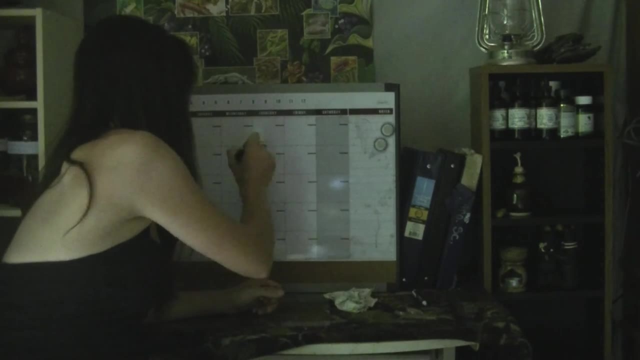 what's called Ovate. Ovate is kind of a cross between the Lancelot and the elliptical. It's kind of gonna be like a triangle, but with all curved edges: The tip is curved, the bottoms are curved, etc. That's called an Ovate After Ovate. 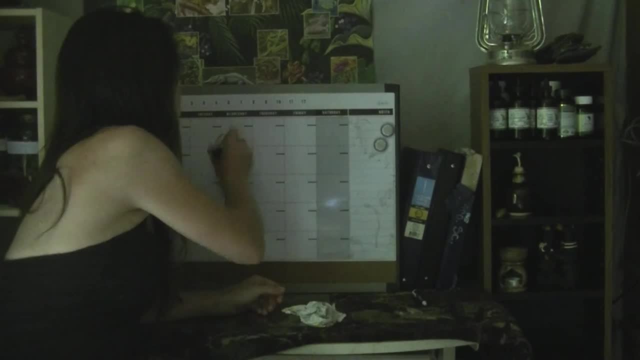 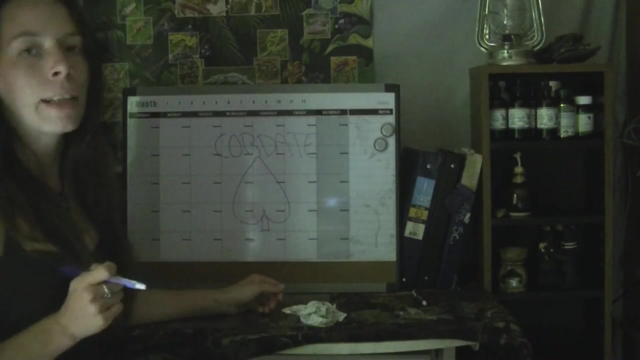 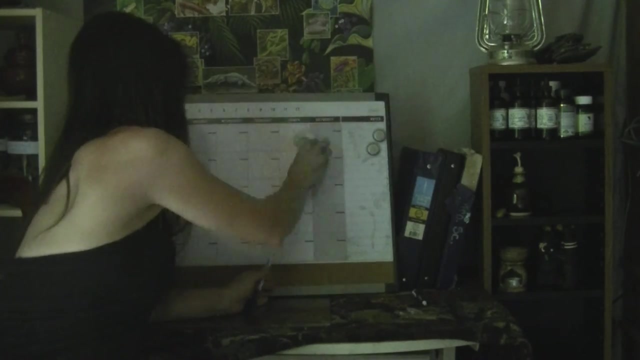 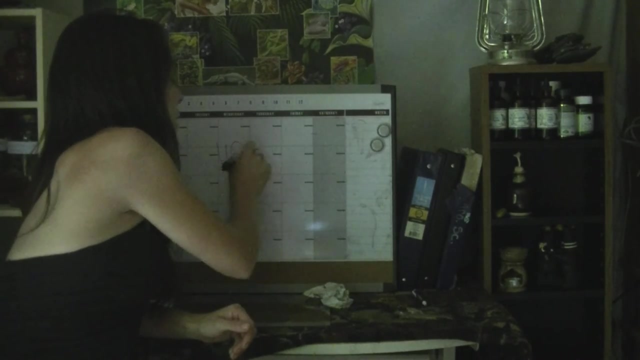 you have what's called Chordate. Chordate is your upside-down heart-shaped leaf and your petiole would be coming out of the base of the heart. That's called your Chordate. After Chordate, you have what's called a Hostate. This is an awkward shape plant. 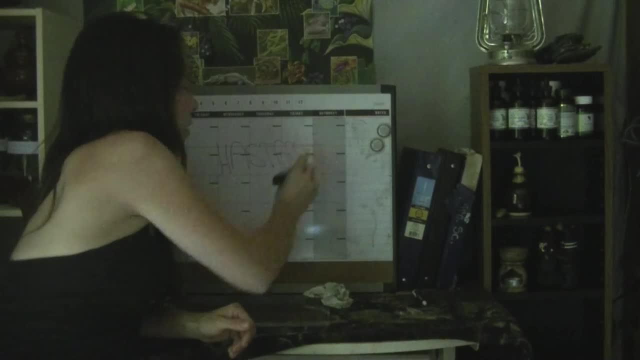 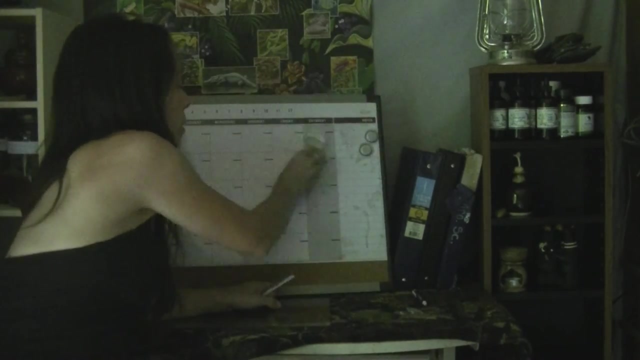 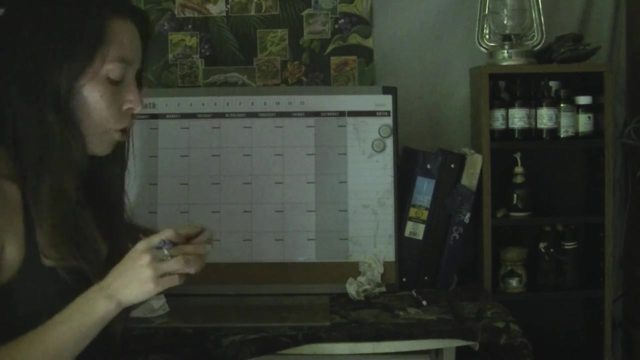 or leaf. excuse me, They're gonna kind of have one spear coming out the middle and then one coming out each side, Just like that. That's called a Hostate, And then the last one we have is what's called Linear. Linear is just like the ovate, except for much longer. It's a very long, skinny, oval-like shape. 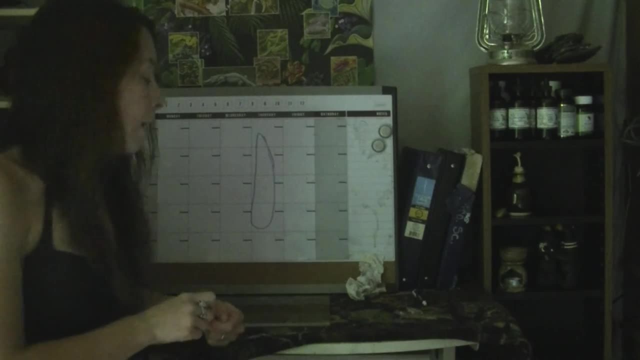 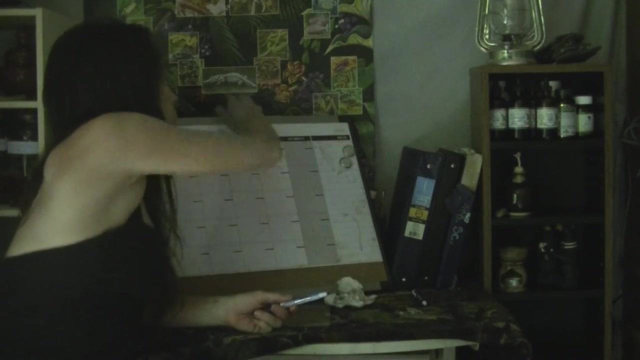 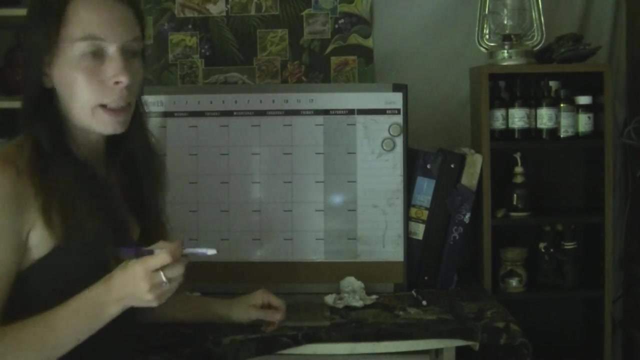 usually at least twice the length, as the width is going to be your linear. If you can identify them by the shape, you can always identify them by the way that the veins are shaped. Veins that are linear means that they're all, if I have my leaf here. 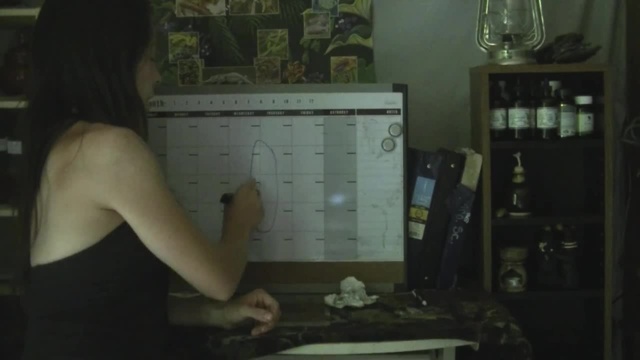 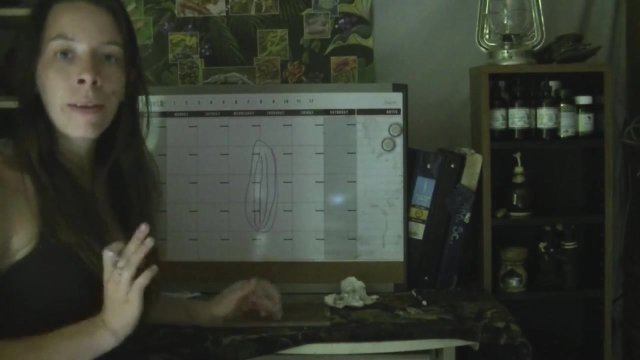 all your veins are going to come from the base of the plant and run the same length all the way up the leaf. So that's called linear: the same length, coming from the same point at the base of the leaf and running up the leaf alongside of each other. so they are. 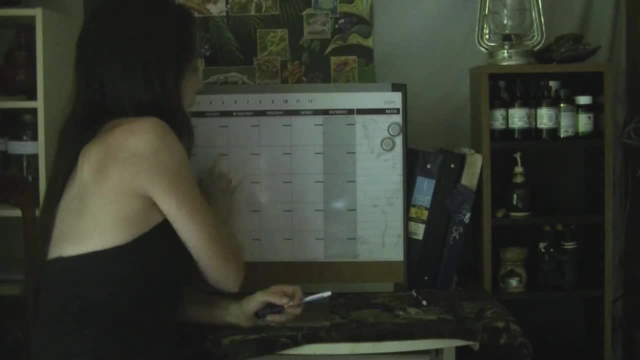 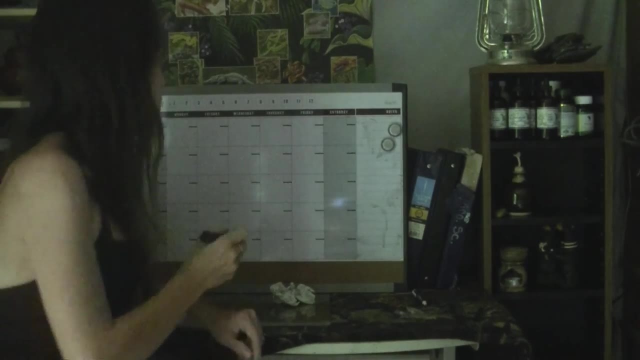 linear. If you can identify them by the shape, you can always identify them by the way that the ear. Then you have pinnate, which is just like the compounds we were talking about earlier. that's where it comes from. is the pinnate, which means that you have 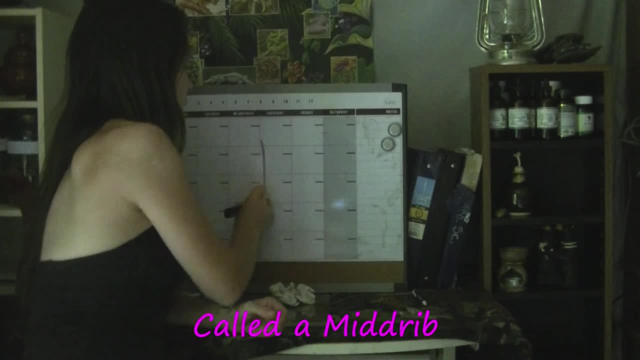 one center vein and then all your other veins are coming off that one center vein, just like how the leaves grow when they're pinnate. So that's a pinnate vein. Then you have what's called a palmate vein, which is, again, is just like the. 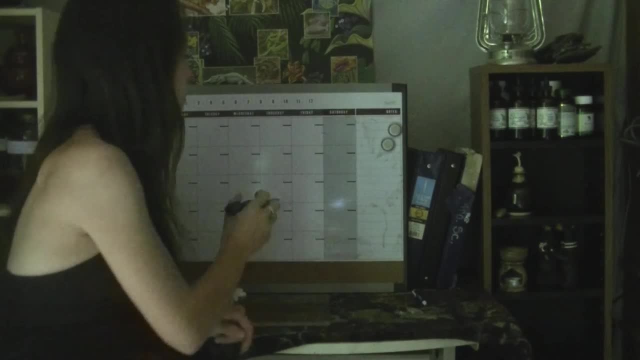 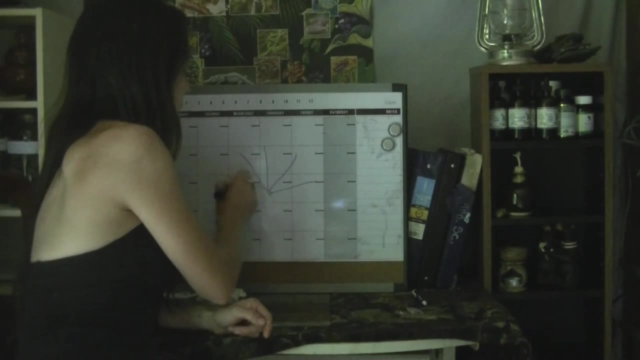 compound of leaves we talked about. when it's palmate, That means that it has multiple central veins. they all come back to the same point but they run in different directions, are different sizes and often time have smaller secondary veins coming off of the main veins. That's called a palmate. 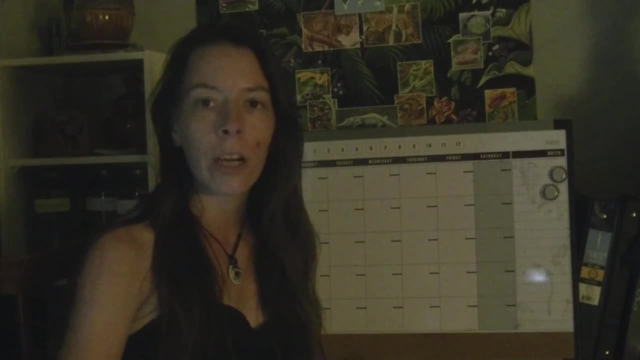 Alright, guys, the very last thing I want to talk about before we leave is specialized leaves that do not fit into any of the categories that we just spoke about Mainly. I just think it's pretty interesting. The first one I want to talk about is what's called a bract A. 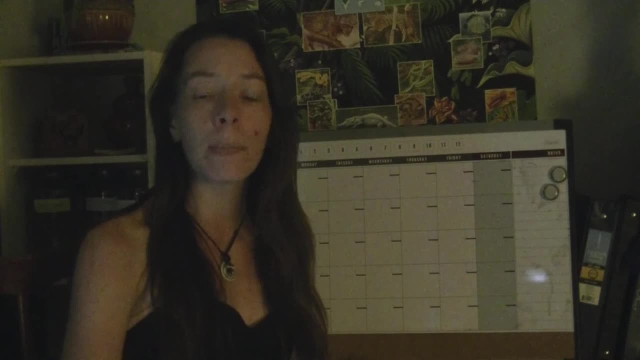 bract is B-R-A-C-T, and these are specialized leaves that act as helpers and defense mechanisms. The best one that I can think of to give you for an example is a poinsettia plant. Those red flowers that you see on them at Christmas time are not actually. 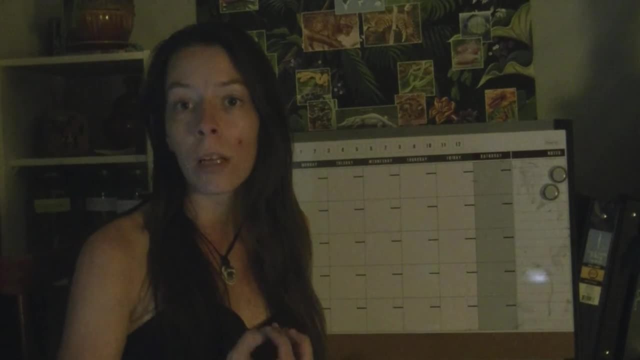 flowers. Those are leaves, and the flower lies in the middle of those leaves. So what these specialized leaves do is they either produce colors and patterns that attract pollinators to the flower, or they repel predators to keep them from eating the flower. Another one that I want to talk about is what's called a 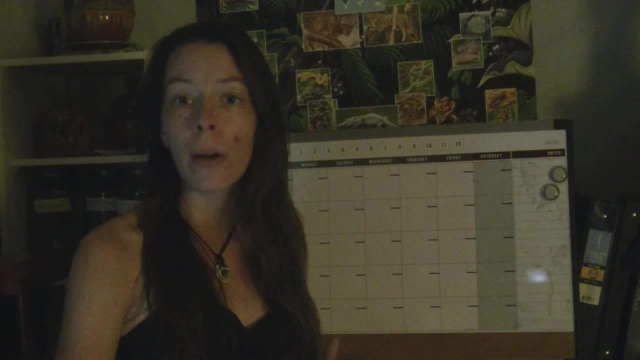 reproductive leaf. The best example I have is a spiderwort plant. These are leaves that actually do the reproduction for the plant. They'll start growing a new little baby tiny plant off the end of that leaf. It's actually very cool to watch and makes it really easy to propagate those plants. Another one is called spines. These are a defense mechanism. Thorns on plants and the spines that are on cactuses are actually scientifically classified as specialized leaves. Another one is your succulent leaves, A good example. 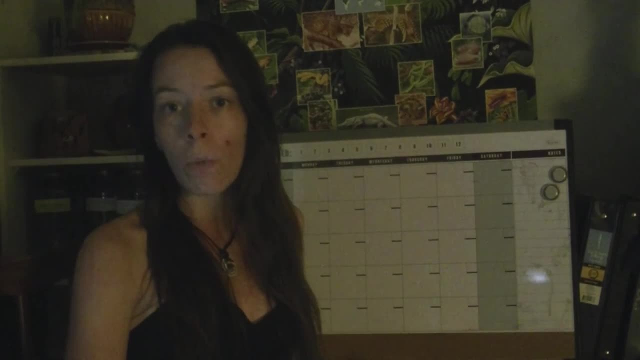 of these are aloe vera. I also did another one on in one of the Shenandoah videos we just made, where we found some Allegheny stone crop. That's also a succulent leaf. These leaves are very thick and they almost feel like rubber. 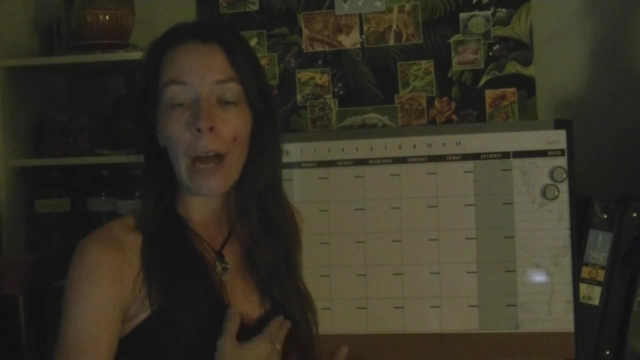 Those are used to store mass amounts of water to help protect plants living in harsh conditions, Things in windy, cold areas, things that have to make it through winter time, etc. Those are called your succulent leaves. Um, another one is called your tendrils. When you have a vine plant, such as your peas, you 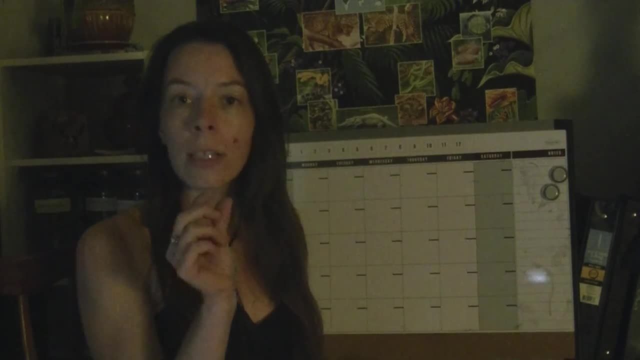 have your main vine And off of that you'll have what looks like little, mini, tiny- almost- you know barely the thickness of a needle type vines that come out and those are what tie to other plants and tie to your trellises, etc. Those are called tendrils and those are also classified as a type of leaf, And the most interesting one I found is bulbs. When you eat an onion and you pull that up out of the ground, you're not eating a root structure. you're actually eating a type of leaf. Each one of those layers that you can peel back on an onion is 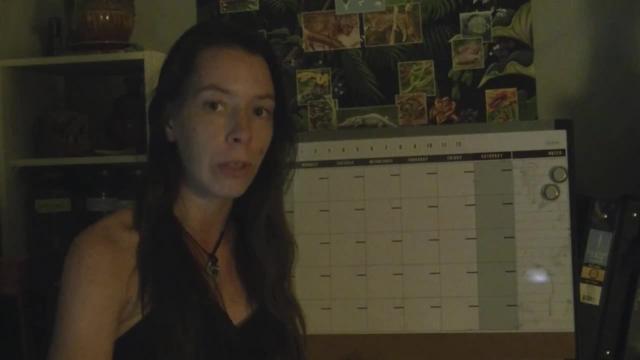 another leaf that's been modified and swollen for food storage. So that's pretty interesting. So those are just a few leaves that you can find and use to be able to determine your type of plant, but will not fall into the categories that we've talked about previously, So I just wanted to let you guys know that also. it's pretty. 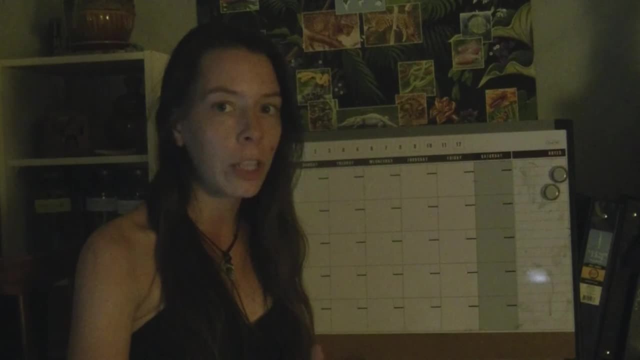 interesting, But otherwise, thank you guys so much for watching. I am going to try to post videos soon that incorporate root structures, flower structures, etc. And we'll go more and more in depth and in detail with how to identify our plants, because it is like I said before. 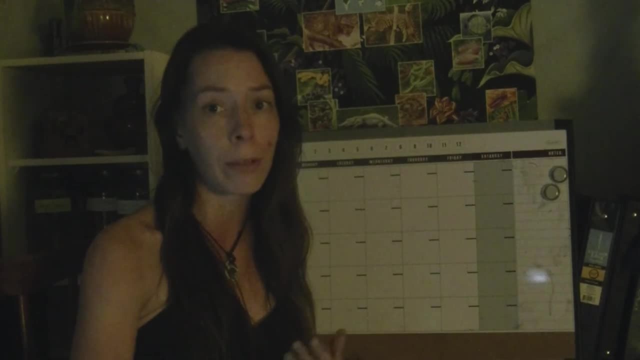 very important to know these things when you're talking about survival or living in the woods or living self sufficiently, And even if you're not doing any of those things, it'll save you a ton of money when you can identify plants, because you can make your own medicines. you. 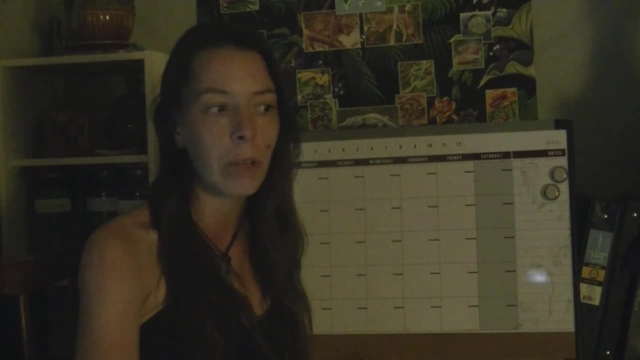 can make your own food. I do quite a few too. I'm going to have some videos coming up on how to make a few different ointments with plants and things like that that I use all the time. that work amazingly. So feel free to definitely comment or message me, Ask me any questions. if there's anything that I didn't go in depth with enough or I didn't explain well enough, or you want to know more, Just let me know. I'm absolutely happy to help. But thank you guys so much for joining me and supporting me and watching. I absolutely love you guys. So enjoy the rest of your day. I'll see you next time. Bye. Enjoy the rest of your day and your time.